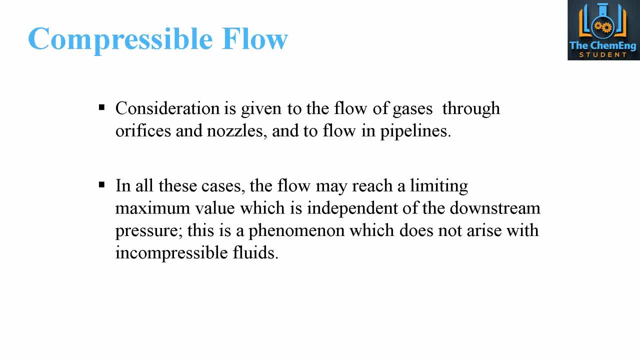 have non-Newtonian fluids that are susceptible to compressibility, But here we're just going to consider gases through orifices, nozzles and pipelines. Now, within each of these cases, we have what's known as a maximum value, which is independent of the downstream pressure. 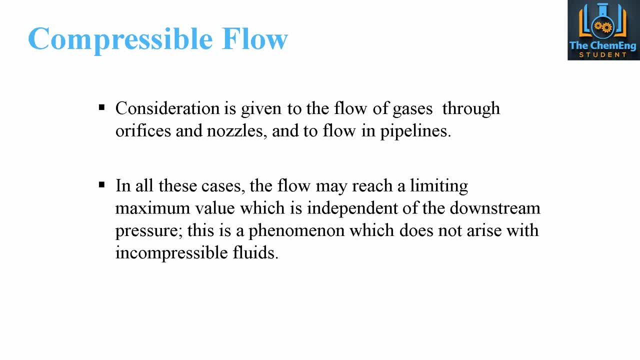 So, up to a certain value of the flow rate, the pressure, the influence that the pressure will have, is negligible. after we reach the maximum value, then this becomes dependent on the pressure of the system, And this phenomenon is what is known as not to arise without a 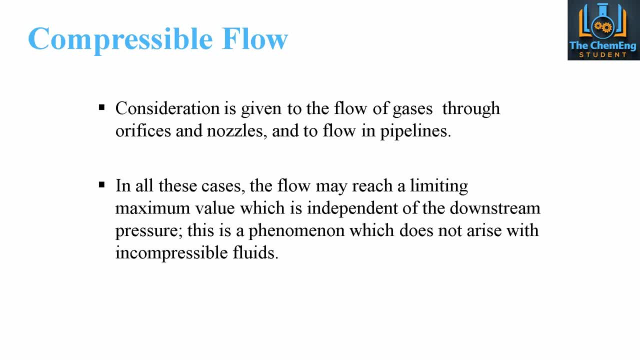 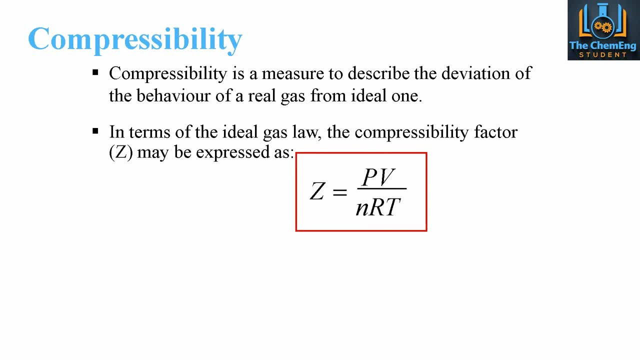 compressible fluid, So this only applies to compressible fluids. Now, the compressibility is a measurement described of the deviation of the behaviour of a real gas from an ideal one, And what we can express this, as is the compressibility factor Z. Now 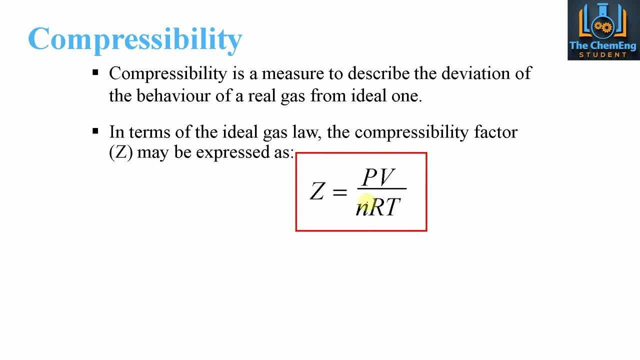 this is in terms of an ideal gas. So Z is equal to the pressure of the system, the volume divided by the holes, multiplied by the universal gas constant, multiplied by the temperature of the system. Now, a very practical example would be in terms of, say, for instance, you're looking at a compressed 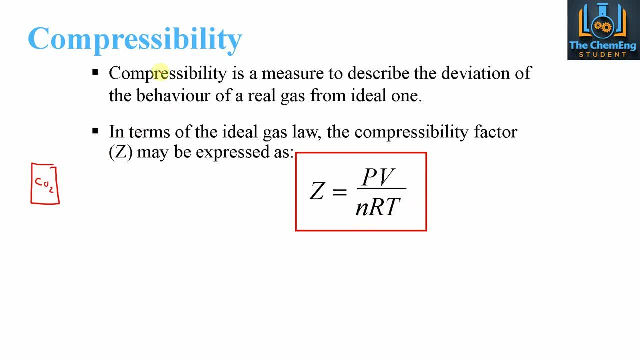 vessel of CO2.. Then usually the manufacturer will give you the mass. So say, for instance here: a standard mass for a cylinder of CO2 was around 34 kilograms. Now we want to know what the volume of the gas is. Now, typically what people tend to do is they take the mass. 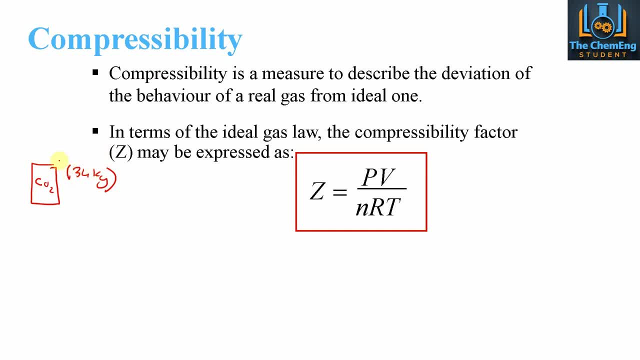 and then they take the density of the system and they can work out the volume, Because, remember, your density would be m³ per kilogram. So what people would do is times by the mass and that would give them the volume. However, this isn't the case, because the CO2 or the 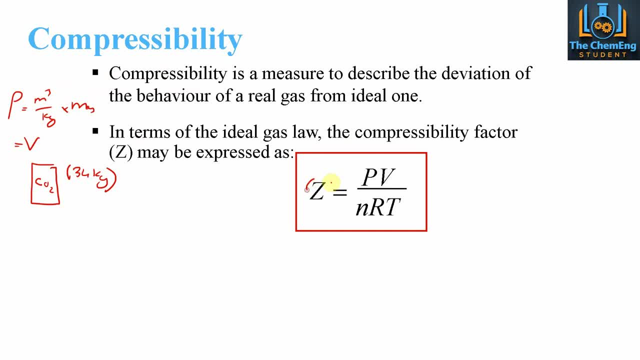 gas compressed. so we need to know the compressibility factor first before we can rearrange this equation in order to find the volume. Now the values of Z for gases are determined experimentally and as such, there are a series of compressibility charts available. Now we have several different references. 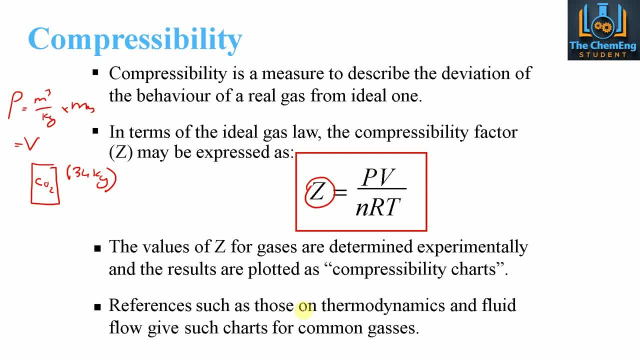 on thermodynamics and fluid flow in our online resource library, so be sure to check that one out, and you can get all your relevant values and data from those charts. This makes life a lot easier when you come to finding and sourcing key pieces of data needed for your problems. 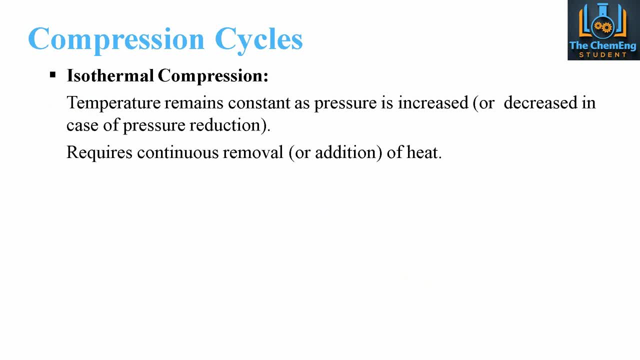 Now another couple of types of compression that we need to discuss here when we talk about compression cycles Now, the first one is the isothermal compression system, and this means that the temperature will remain constant as the pressure increases. Now, the temperature will remain constant as the pressure increases. Now the 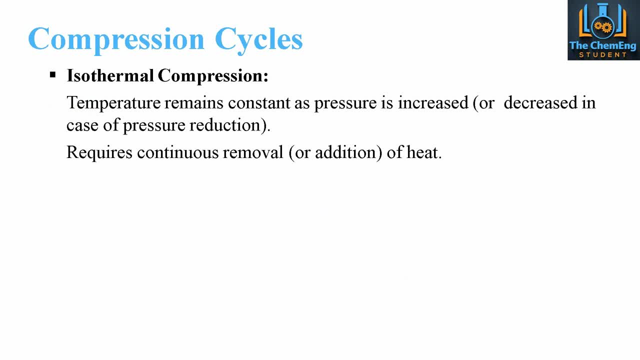 pressure increases Now, the temperature will remain constant. as the pressure increases Now, the temperature which will be reduced is either increased or decreased, and this would therefore require, for isothermal compression, the continuous removal or addition of heat, depending on the system. For those of you, 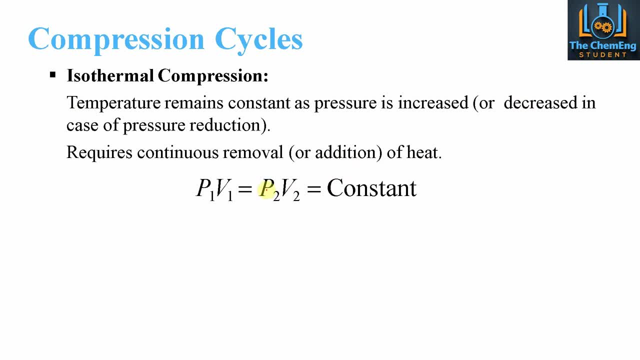 that have done our heat transfer course, our thermodynamics and fluid mechanics courses, you. so we can relate the pressure in the volume at point 1 with the pressure in volume at point 2.. Now the other type of compression is known as isentropic. Now 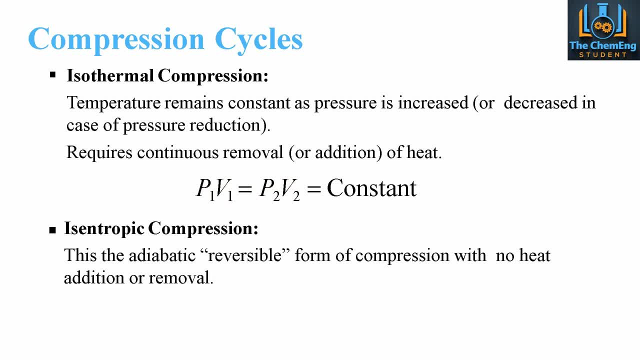 isentropic compression is the adiabatic or reversible form of the compression, with no addition of heat or removal. So it follows the same principle, but because we don't have the addition or removal of heat and the system is reversible, we then introduce this new parameter, gamma. So we have P1. V1 is 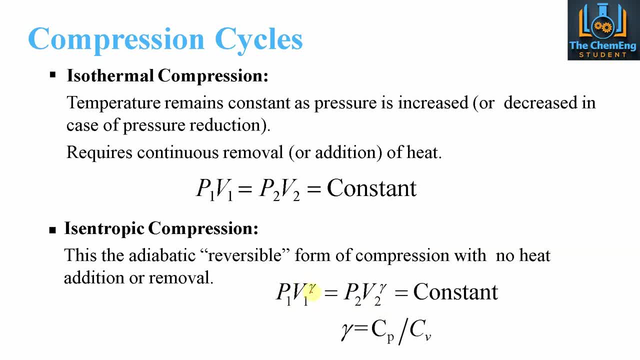 equal to P2, V2, but the volumes are to the power gamma. Now gamma is expressed as Cp over Cv, so it's the rate relationships between the specific heat capacities. Now this is, of course, dependent on your fluid. so gamma can be found through published data for the values of Cp and Cv. Now that's all very.